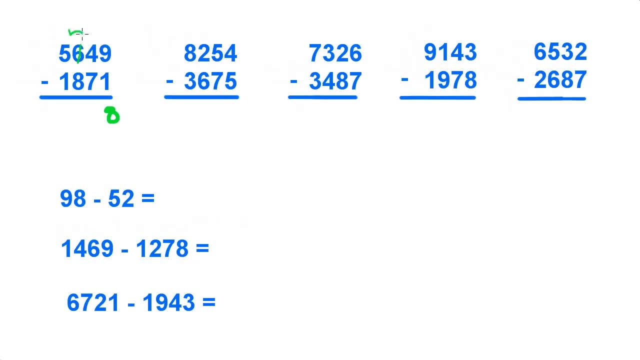 do that, so we have to borrow from the six, make that a five, make that a fourteen. Fourteen minus seven is seven. Five minus eight cannot do that, we have to borrow from the five again, make that a six, fifteen. Fifteen minus eight is seven, and six minus one is five. There's 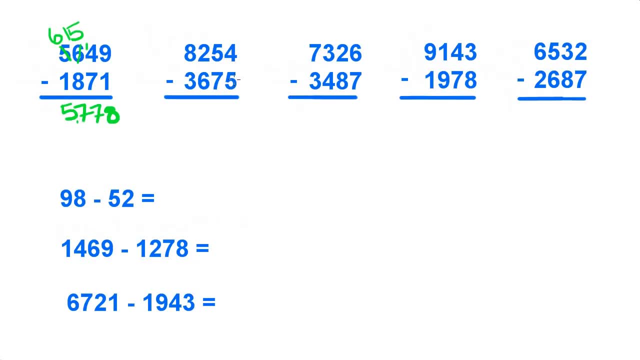 our answer. We start over here, four minus five, borrow from the five, make that a four, put the one right there, making that a fourteen. Minus five is nine. Four minus seven is eight, eleven cannot do it, borrow from the two, make that a one, make that a fourteen. Fourteen 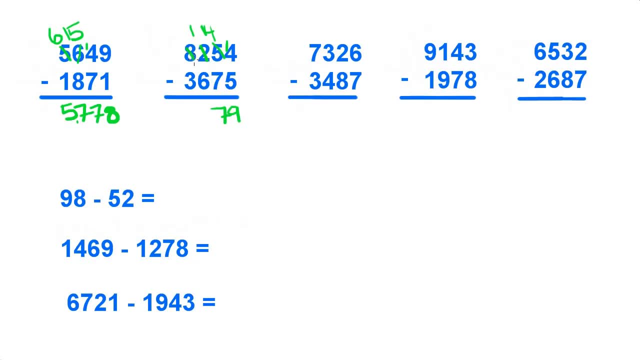 minus seven is seven. One minus six, we have to borrow from the eight, make that a seven, make that eleven. Eleven minus six is five, and seven minus three is four. Over here, we have six minus seven, borrow from the two, make that a one, make that a sixteen. 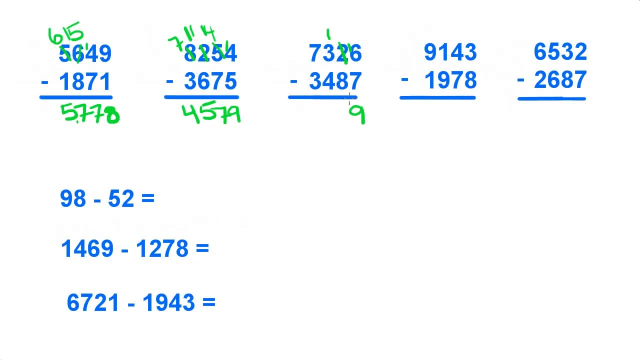 That's going to be nine. Sixteen minus seven is nine, so we have to borrow from the three, make that a two, make that eleven. Eleven minus eight is three. Two minus four, can't do it, borrow from the seven, make that a six, and that's going to be twelve minus four is eight. Then six minus three is three. Over here, three minus eight, borrow from the four, make that a three, make that a thirteen. Eight, nine, ten, eleven, twelve, thirteen is five. Three minus seven, can't do that, borrow from the one, make that a zero, make that thirteen. Thirteen minus seven is six. Four minus nine, borrow from the nine, make that an eight, make that a ten. Ten minus nine is one. Eight minus one is seven. Over here, two minus seven, you need to borrow from the three, make that a two, make that a twelve. Twelve minus seven is five. Two minus eight can't do that.